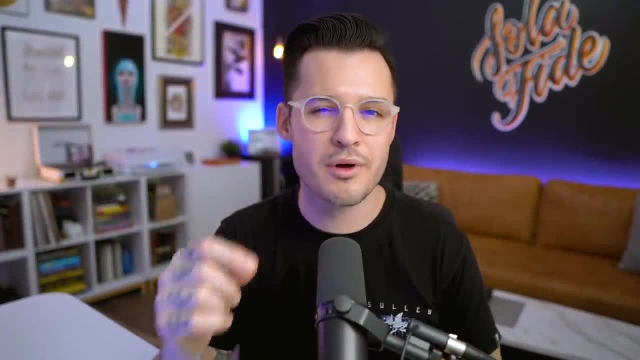 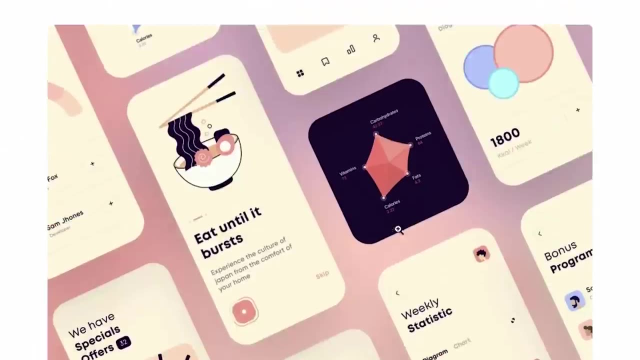 How can you use color inside of your mobile UI design projects that come out looking really mature and really seamless and really well thought out and not obnoxious and loud and really the worst thing that it could be is distracting. Well, you might want to use a. 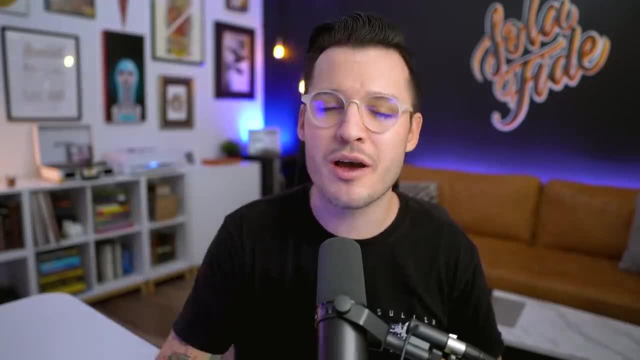 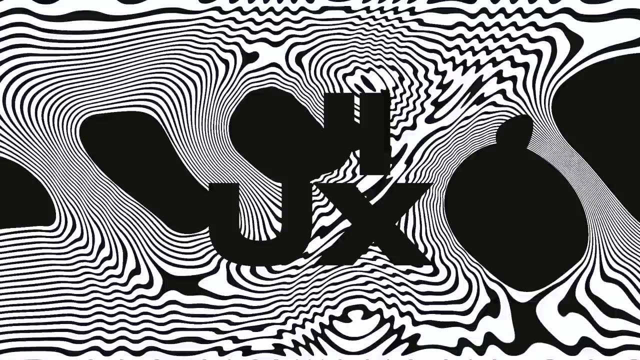 little rule or guideline called the 60-30-10 rule, which is going to help you to understand how to use color, how to implement color and when to break that rule. We're going to talk all about that coming up next. All right, before we get too far into the 60-30-10 rule. 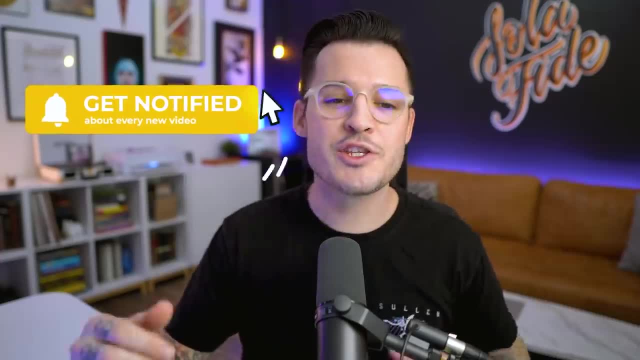 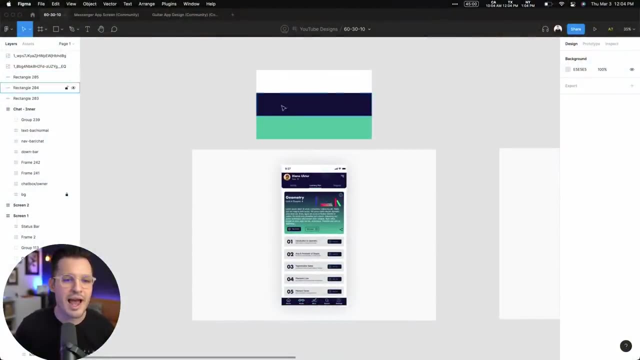 make sure that you like and subscribe to this channel and hit that little bell notification icon so you know when other videos like this one come out. Let's jump over to Figma, so we can talk a little bit about the 60-30-10 rule. I have an image that I pulled from a great blog post that 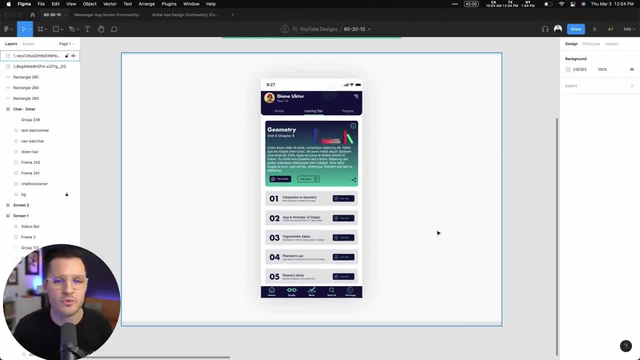 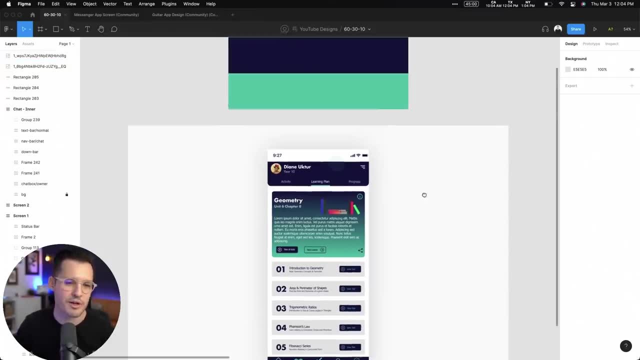 I'll leave a link in the description by a designer who's talking about the 60-30-10 rule and she has a really great contrast and comparison of before and after I'm going to talk a little bit about. I thought it'd be a great use case or case study for us, but I've taken that initial UI design that. 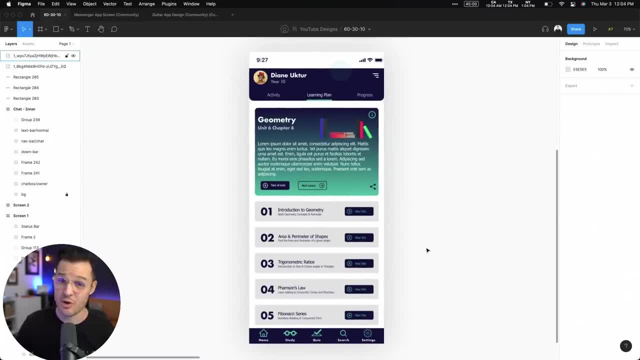 she shows in her post and it's man. it looks like a yard sale. It is really immature. The usage of color is just distracting. It's overbearing. I don't know where I'm supposed to look or where I'm supposed to go. Let's make a little bit of sense with this. in our 60-30-10 rule. I have three. 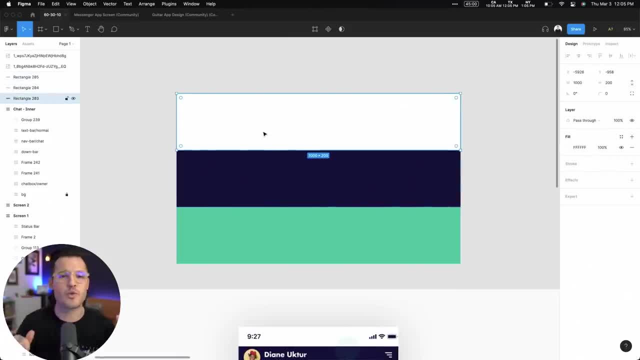 blocks of color up here and each rectangle is 1,000 pixels wide, which represents our 100% of color usage. In our 60-30-10 rule, we want to make sure that we're using 60% of our neutral or our base color. 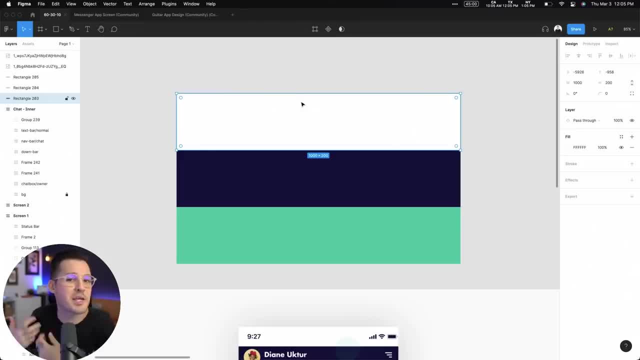 It's going to be a neutral color. It could be a creamy color, a white color. If you're doing a dark interface, it's going to be some sort of dark color Now. later on we'll talk about how you can. 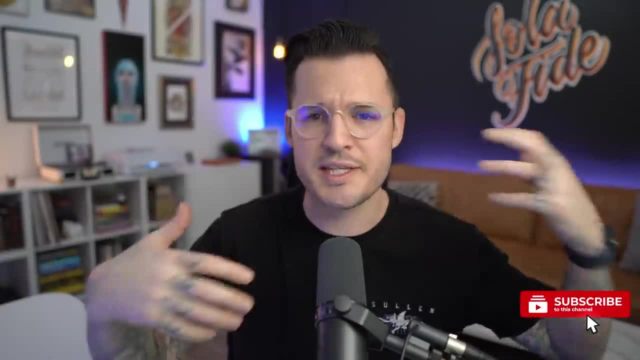 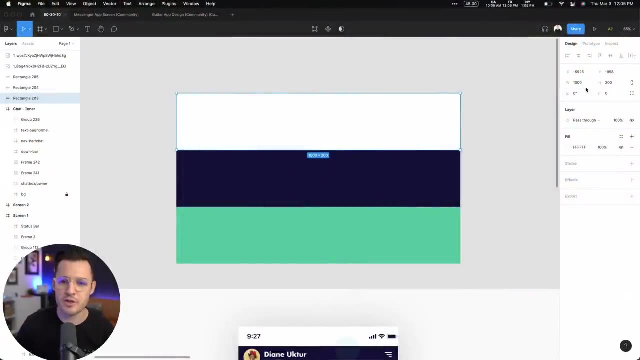 flip this around and do really bright interfaces and use 60% of a brighter color, but for now let's stick with the more neutralized version. 60% is going to be this color, so let's just take this really quickly and type 600 pixels. That represents our 60%. Then you're going to 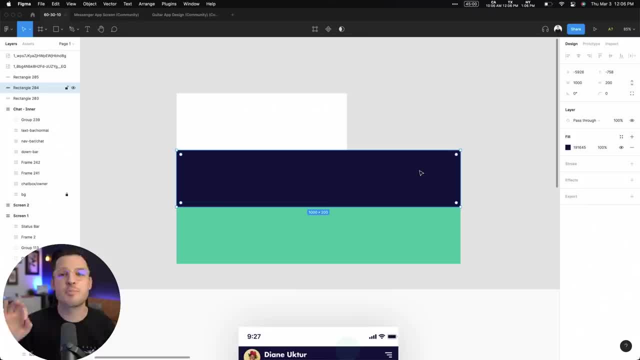 have some sort of primary color, right, This might be a brand color. This primary color is important, but it's not going to be as important as our call-to-action color, our secondary color, This one. we want to be 30%, so let's do 300 here and we'll just pop this up into place. and then, you guessed it, Our. 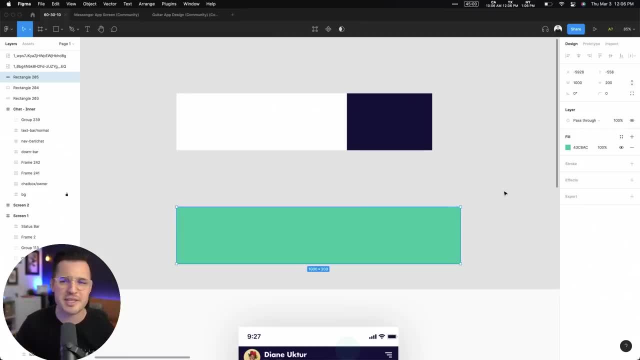 call-to-action, it should be used sparingly. our secondary color: This is the thing that says: click me, look at me, I'm active, do something with me. We want that to only be 10%, so let's take it down to 100, and now we have a color palette that we can use for our secondary color. 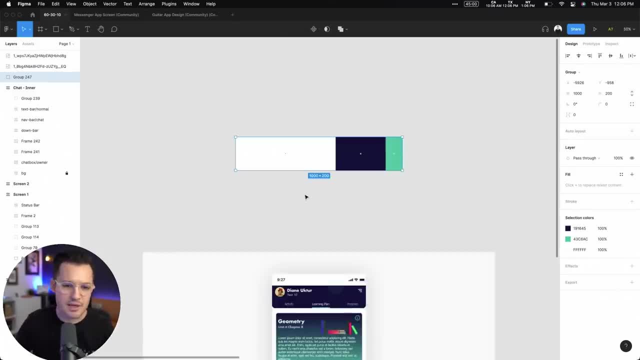 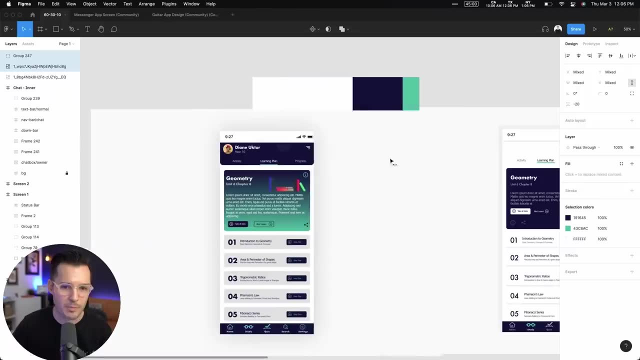 We can use for 60,, 30, and 10, and you can see this- 60,, 30,, 10 is not well represented in this version of the design, but I would say it is much more represented in this next, this iterated. 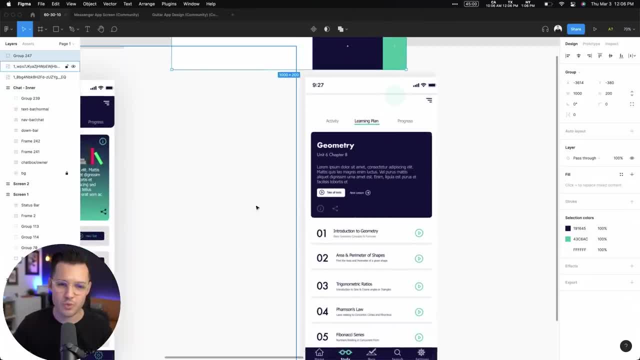 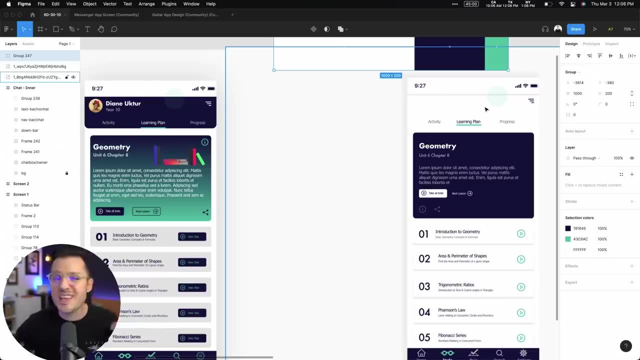 updated version of her design. where she's now, she's really like done away with a lot of the excess use of color. She's stripped it down. She's kind of neutralized thing. Now, yes, there's some other fixes here, some copy fixes, some iconography fixes. but even if you kept all, 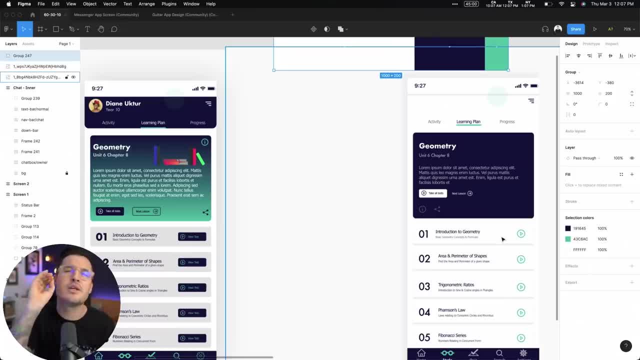 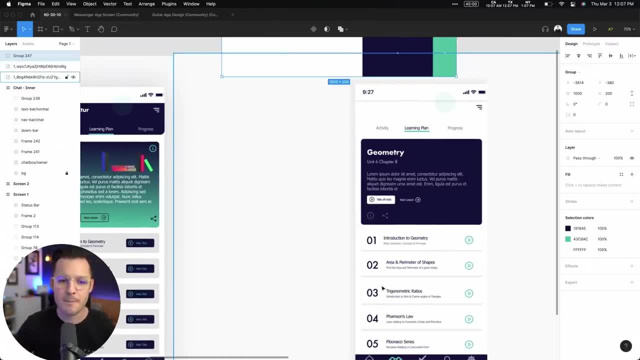 the other colors. you're going to have a lot of color. You're going to have a lot of color. little mistakes in this previous design. The color is just heads and shoulders, heads and tails, whatever you want to say. a much better version of color implementation here, Much more neutralized. 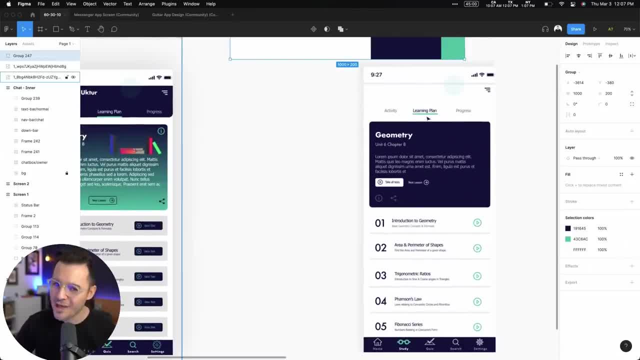 here, right, Our primary color is being used for important areas and our call to action color is only in very important areas. Click me, do something with me, pay attention to me. This is for you. user these call to action areas, and so that's the 60, 30, 10 rule. Let's really 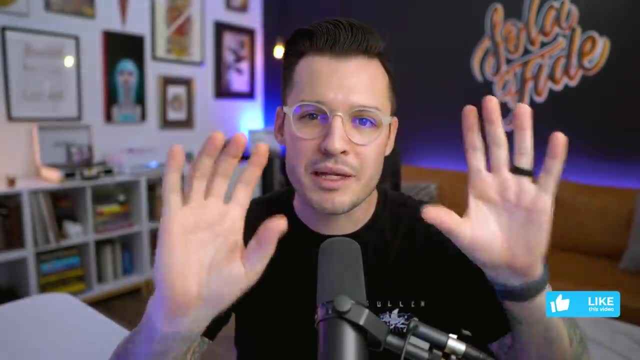 quickly take a look at some other implementations of the 60, 30, 10 rule. Let's take a look at some of the 60, 30, 10, but keep in mind it's just a guideline. I'm going to show you some great. 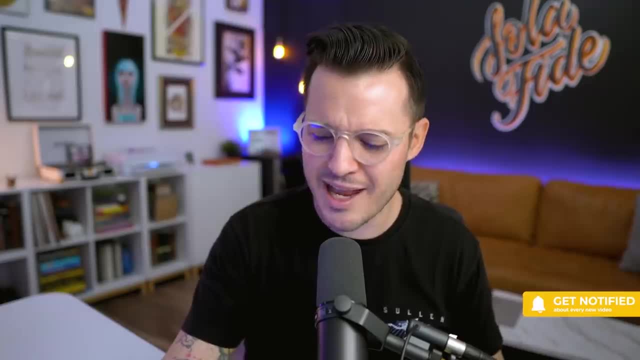 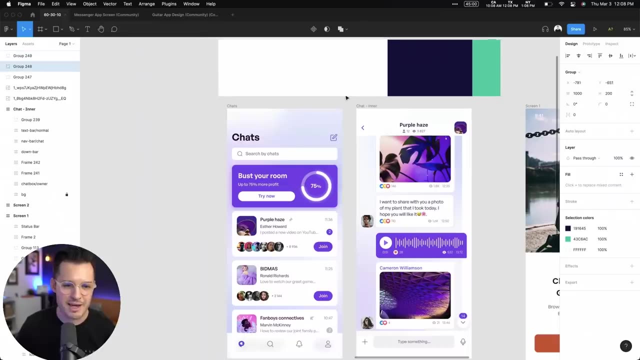 kind of uses of 60,, 30,, 10, but they're breaking it a little bit and that's okay with me. It should be okay with you as well. I pulled some Figma community files in here. Now you might say: 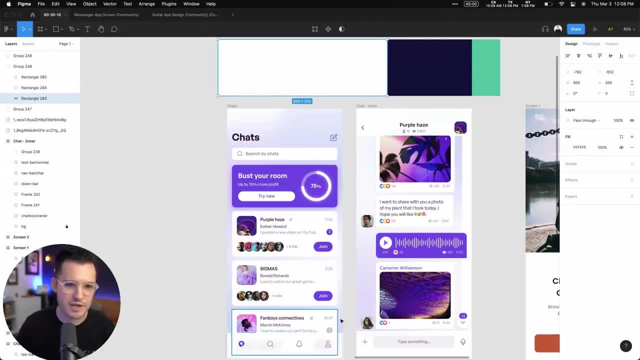 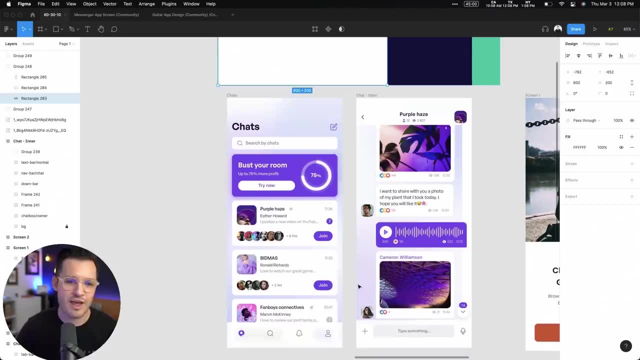 that this neutral color is, whatever this kind of like grayish color is That works. Oh, it looks kind of like white, but it's not really. but maybe it is white, That's fine. And then you might say that your secondary color right, and they're breaking it a little bit. 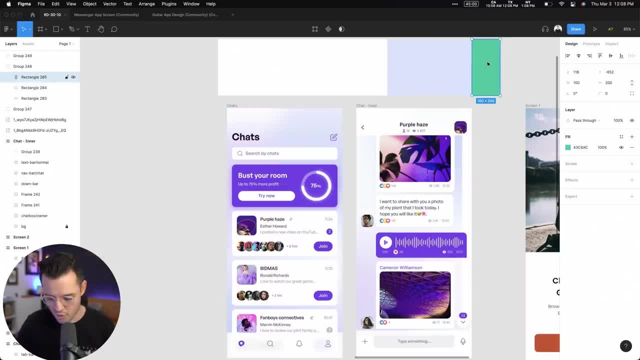 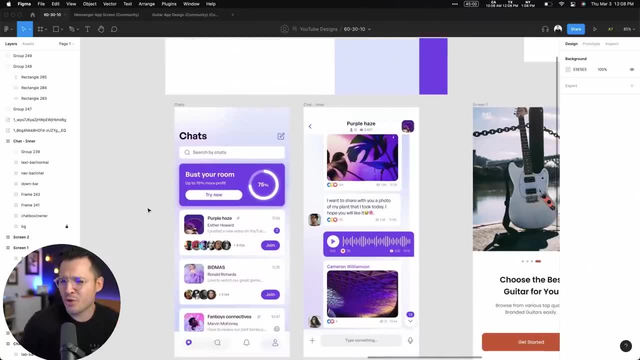 is maybe kind of like this bluish color and then your- excuse me, your primary and then your call to action color is definitely this kind of purpley color, but that's still kind of 60, 30, 10.. They're throwing some fun gradients in the top and playing with it. 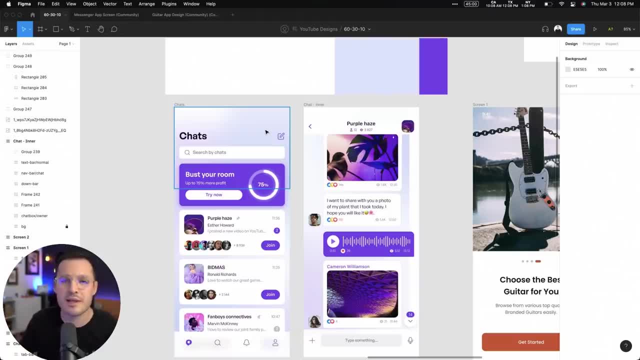 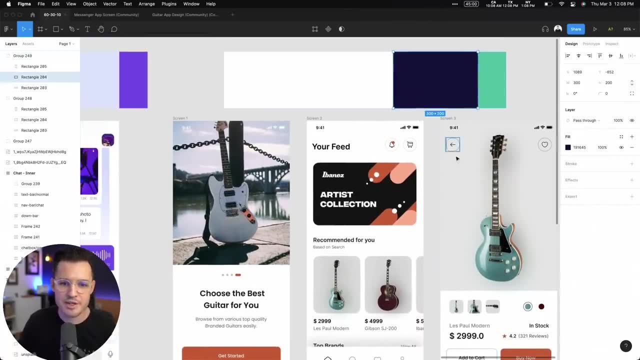 but I'd say this is more of a two-color design and they're just kind of utilizing some hues of that color. Let's do this one over here by Mohit Designs. We got a really similar thing happening. We got white right and then you're going to see throughout over like kind of a span of multiple. 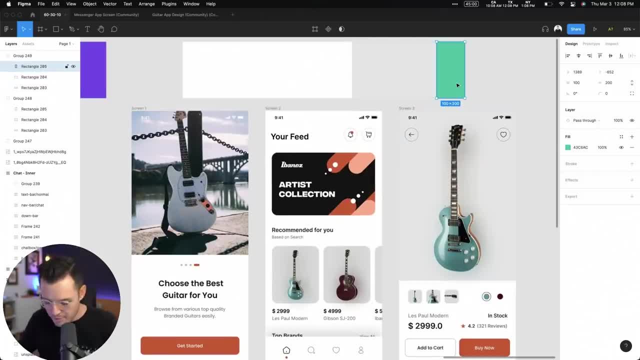 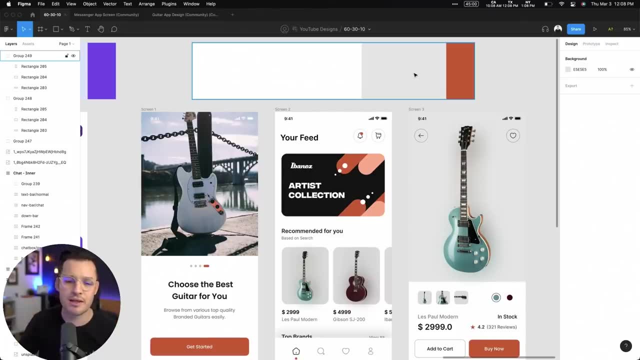 screens that maybe our primary color is kind of this gray but that call to action color is really this kind of warm, kind of burnt orange color, We can see a really beautiful color palette. So it's just a good usage of the rule in UI design. Let's look at a couple more examples. 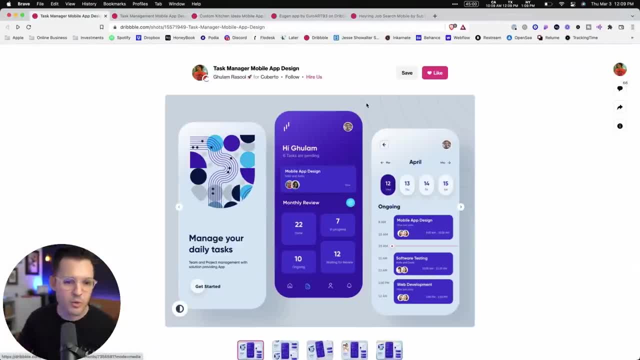 online. Here's some great examples on Dribbble. This one by Ghulam Razul. This is an example of kind of the reverse of it, where your bright color is 60% right and then you can see we have 30%. is a lighter hue, So that's kind of a good usage of the rule in UI design. Let's look at a couple more examples online. Here's some great examples on Dribbble. This one by Ghulam Razul. This is an example of 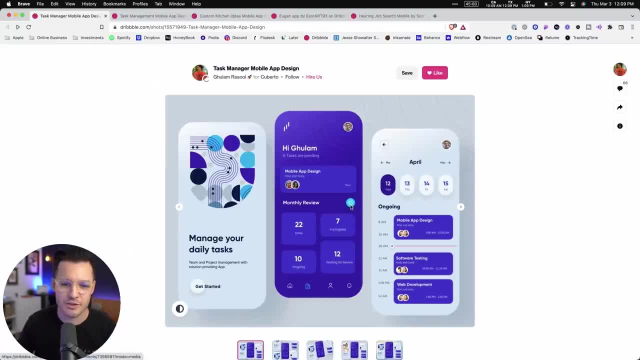 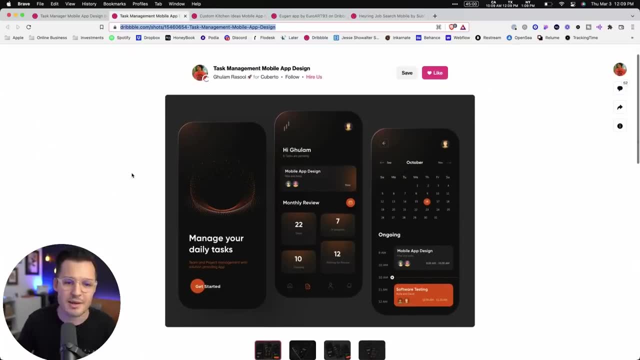 but look, still 10% on the actionable colors. We're still doing the 60-30-10.. We're just using color instead of a neutral. That's okay, I'm down with that. Here's another one by the same designer. 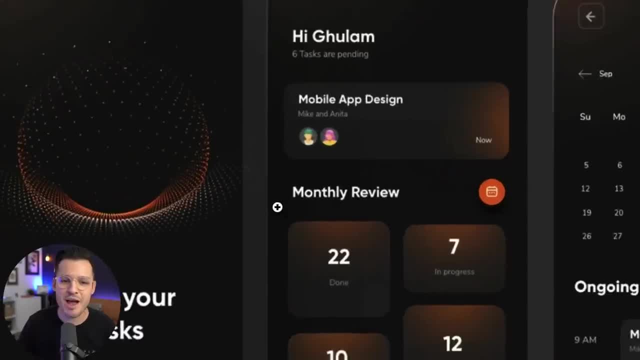 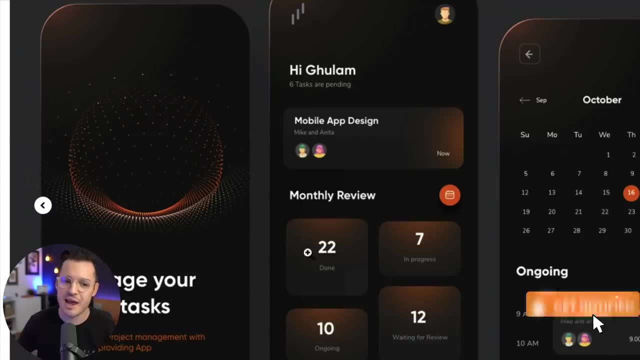 He's just kind of like flipped it to a dark interface. Look same kind of like guidelines even in a dark interface. 60% is going to be this real dark color, 30% is going to be these lighter colors. He's bringing some gradients into them. That's fine with me, but only 10% is being used. 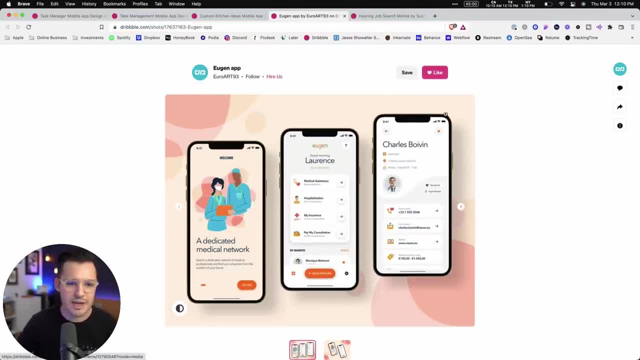 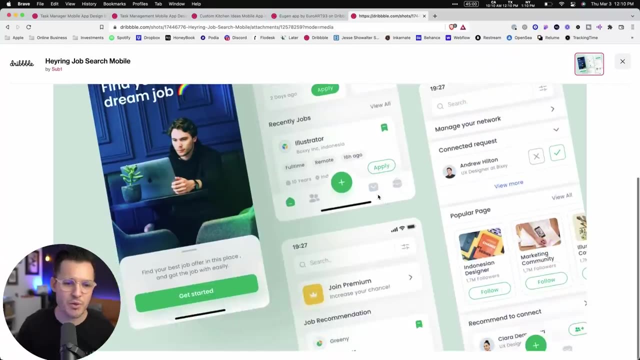 for that accent color. Let's take a look. Let's do another one by EuroArt93.. Again, we zoom in, We see 60%, right, 30%, 10%. And last one, just to drive the idea home one more time. This one is by Sub1.. This beautiful little bit of UI.